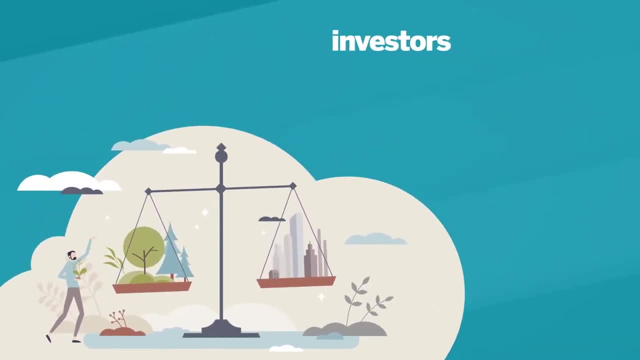 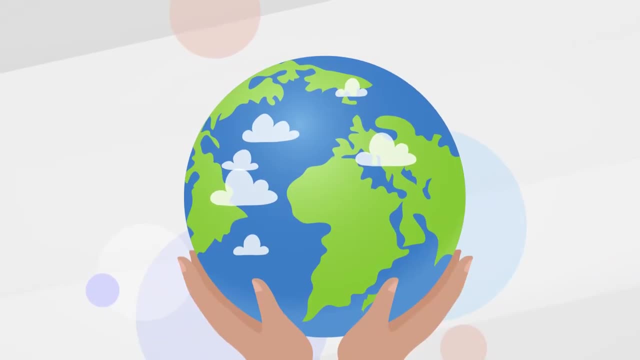 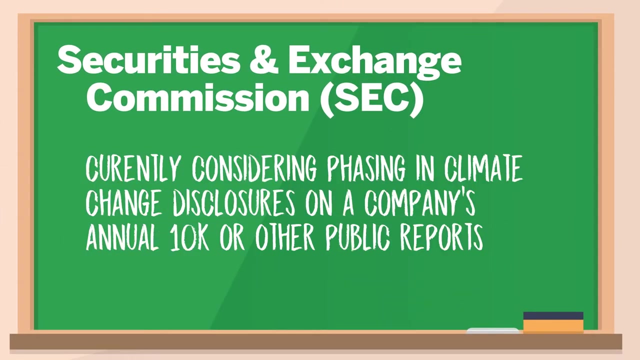 Companies are accountable to multiple stakeholders, including investors, customers, employees, government and non-governmental organizations who want to evaluate a company's impact on the world. In fact, the US Securities and Exchange Commission, SEC, is currently considering phasing in climate change disclosures on a company's annual 10-K or other public reports. 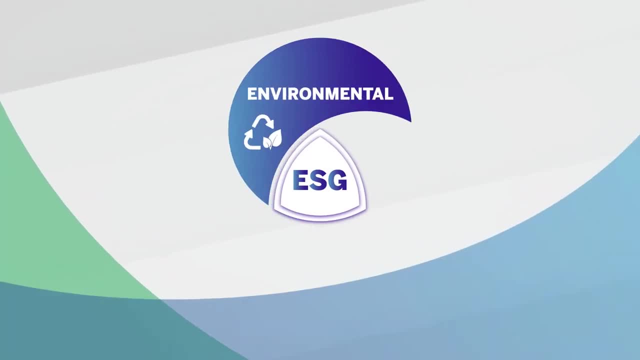 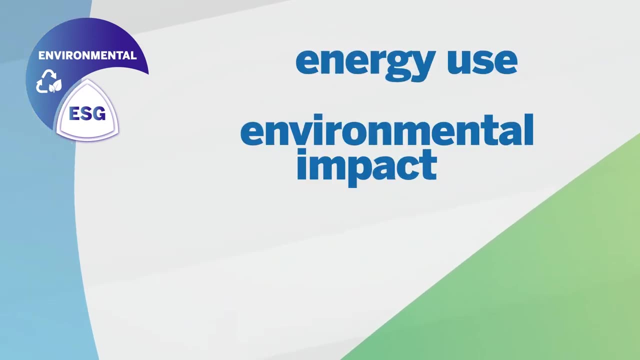 Let's take a closer look at ESG, starting with E environmental. This considers companies' energy use, environmental impact as stewards of the planet, and how a company uses resources across the board, specifically scopes 1,, 2, and 3.. 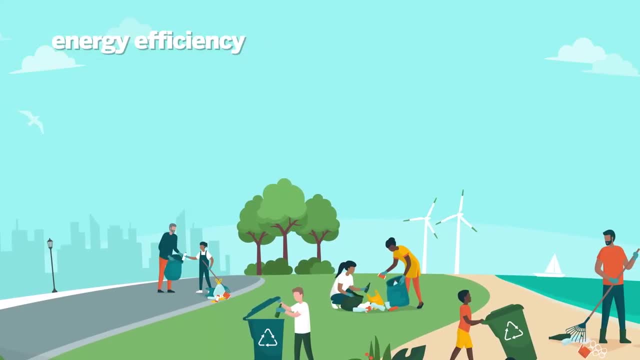 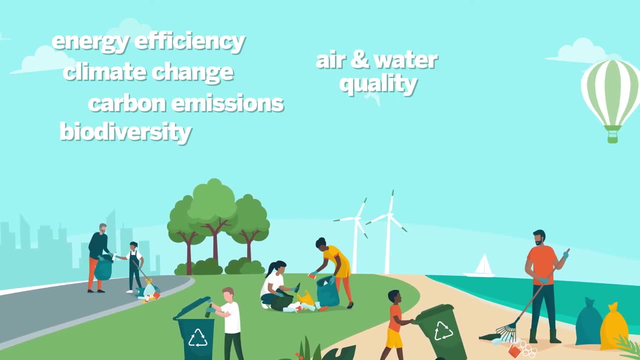 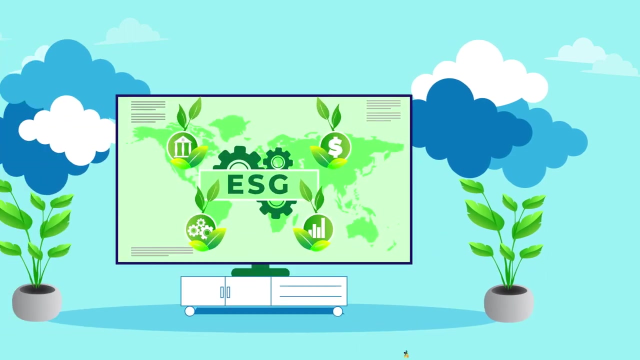 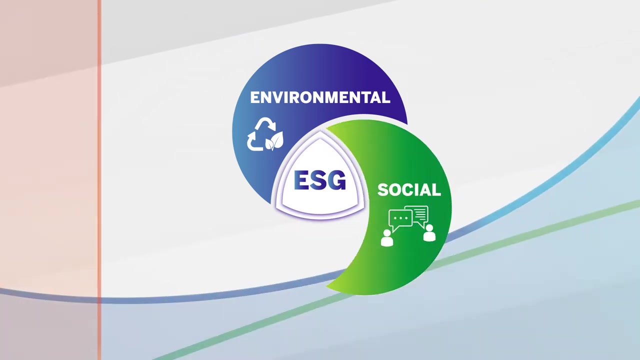 Emissions sources. Factors considered are energy efficiency, climate change, carbon emissions, biodiversity, air and water quality, deforestation and waste management. Organizations that do not consider these environmental risks may face unforeseen financial risks and investor scrutiny. Social: The social criterion examines how a company fosters its people and culture. 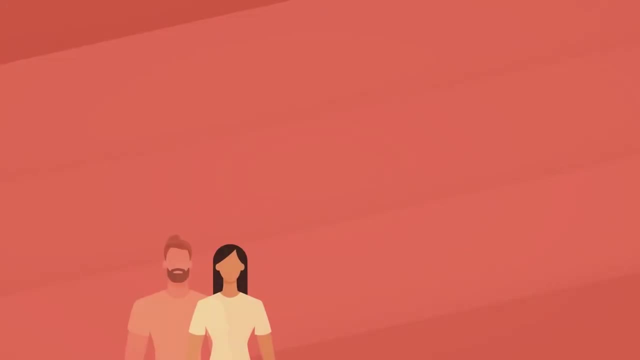 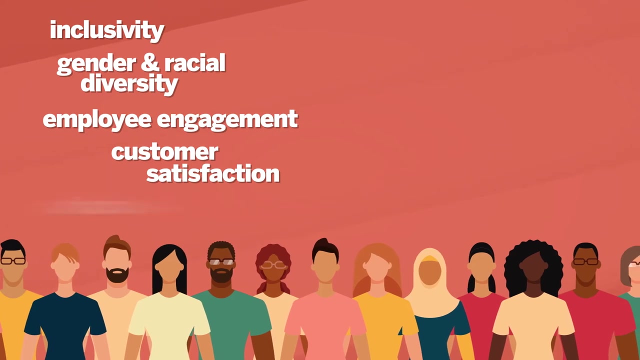 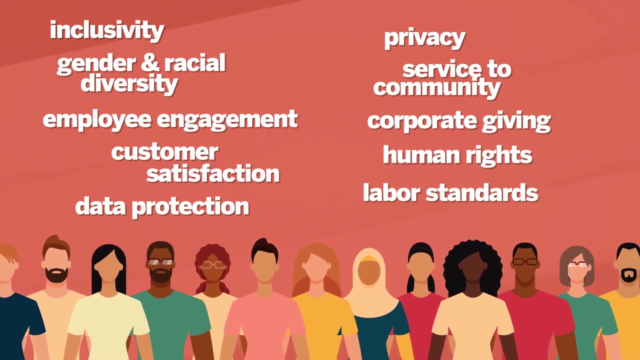 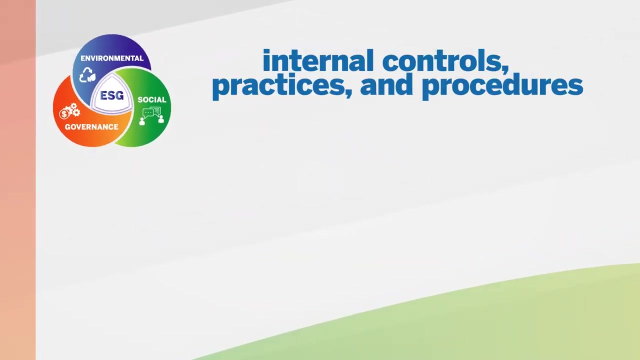 and how that has ripple effects on the broader community. Factors considered are inclusivity, gender and racial diversity, employee engagement, customer satisfaction, data protection, privacy, service to community corporate giving, human rights and labor standards. Governance: Governance considers a company's internal system of controls, practices and procedures and avoidance of violations. 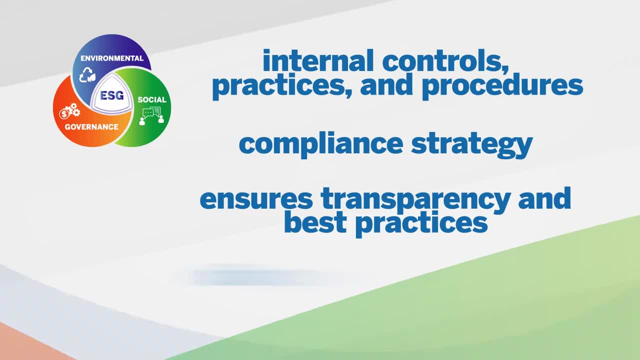 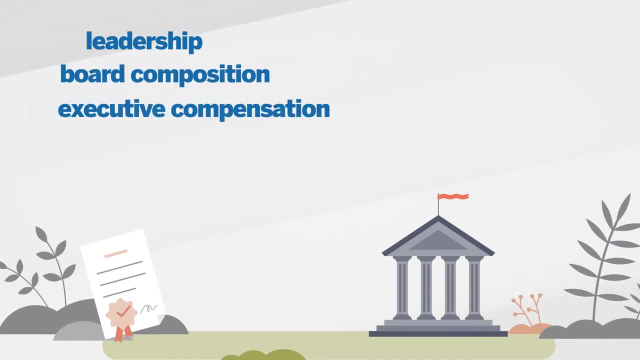 It ensures transparency and industry best practices. It ensures transparency and industry best practices. It ensures transparency and industry best practices and includes dialogue with regulators. Factors considered are the company's leadership board composition, executive compensation, audit committee structure, internal controls, shareholder rights and political contributions. 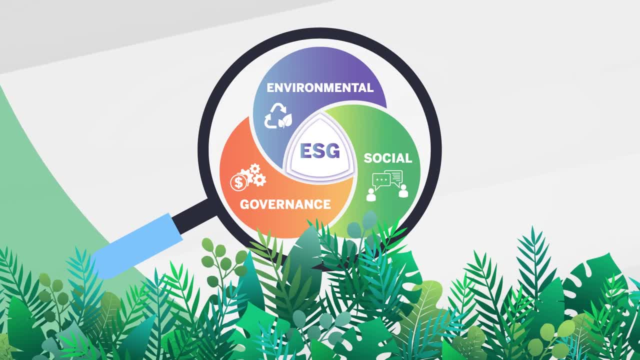 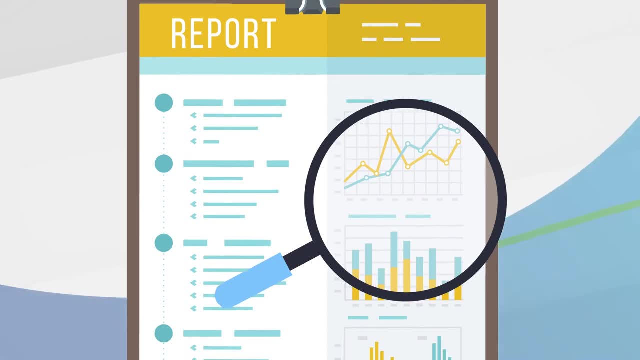 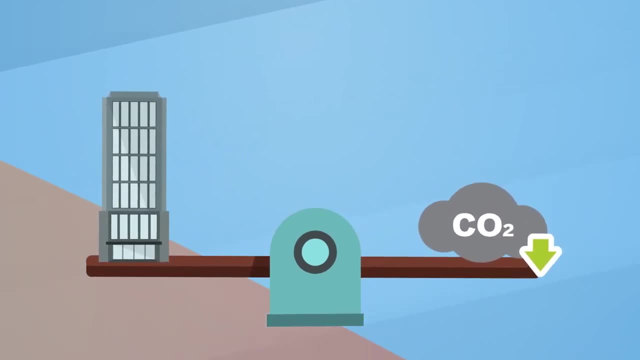 Transparency is critical to the process in which some companies emerge as sustainability leaders, others as laggards. Transparent reporting enables stakeholders to gain a clear picture of a company's direction progression. For example, a company might not be carbon neutral today, but may be. 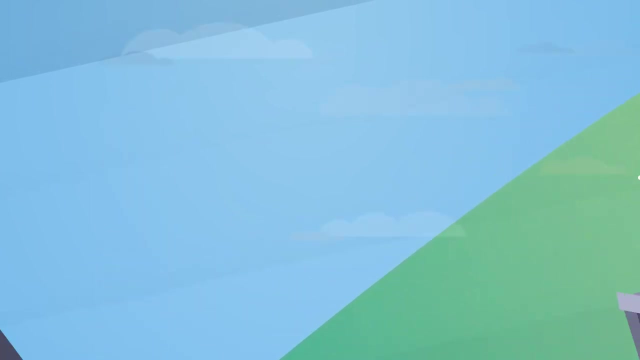 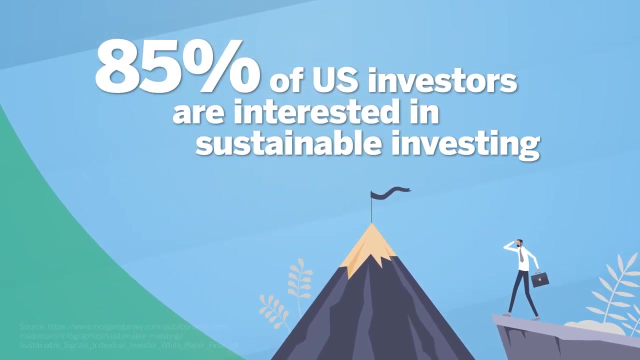 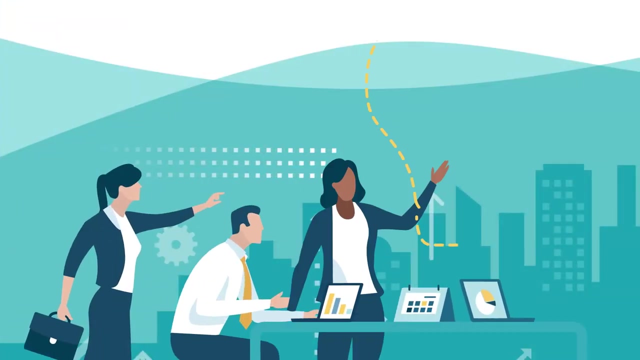 making significant efforts towards this goal. Stakeholders need visibility on the progress as well as the goals. A recent Morgan Stanley survey found that 85% of US investors are interested in sustainable investing. ESG analysis and reporting is becoming more prevalent, Incorporating your values and concerns.